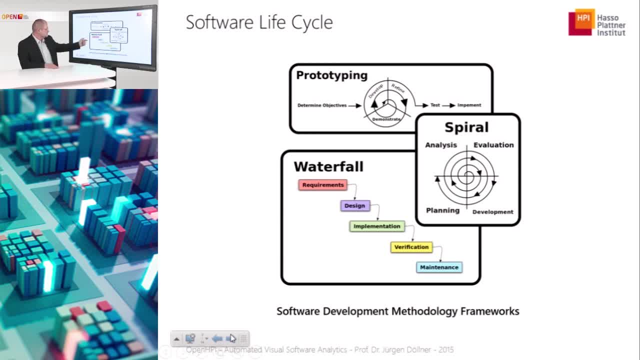 It defines a number of stages: requirement analysis, software design, software implementation, verification and test and finally, maintenance. It defines these stages and they are ordered in a linear way. So software should have a framework, It should be developed by handling all these stages and, as a result, the software should be operational, fully functional and it should have certain software qualities. 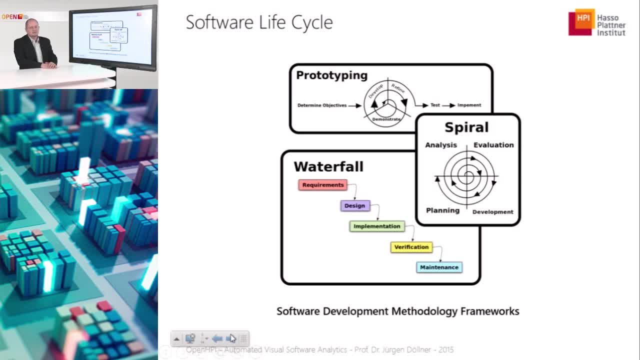 Of course, the waterfall model is a traditional model and not really up to date, because during the last decades we find out that software development has a more dynamic nature. This dynamic nature is represented, for example, in the spiral model. It says basically: we start with analysis, evaluate our design, develop implementations. 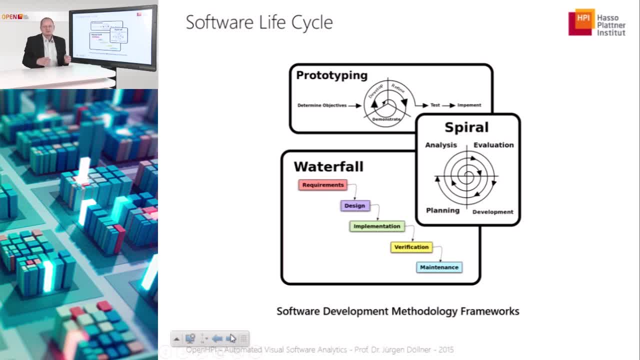 and we do further planning for the next cycle, for the next iteration. There is also a key method around that aims at rapid prototyping, At prototyping software systems. we determine our objectives, develop, refine and demonstrate And we end up with testing and implementing artifacts. 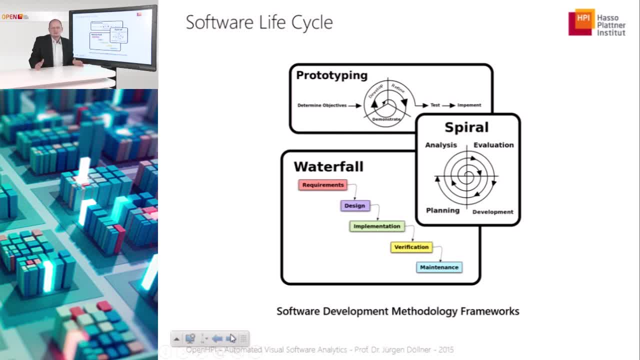 So there is a large collection of methodology frameworks around, And maybe in your team, in your project, you have defined which one you take. There is not a unique or best practice model around, Although today many software development teams use agile methods or scrum techniques. 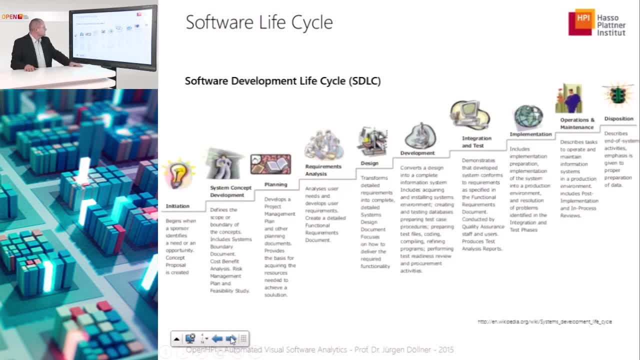 During the software development lifetime or life cycle. regardless of the concrete methodology you are using, we can identify certain stages in all these frameworks. It's the initiation stage, when we begin and we want to identify needs. The concept stage, where we start Sketching and forming models of our software system. 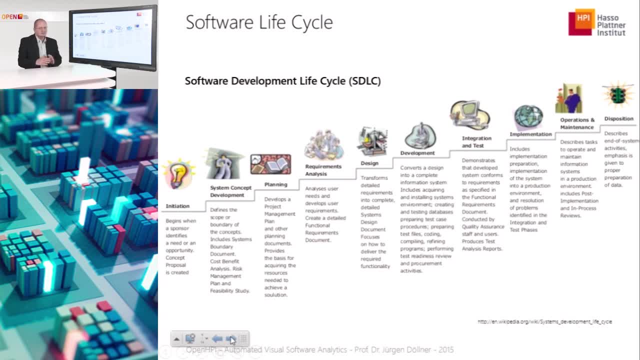 The planning stage, where we start to make more precise models, specifications, requirement analysis, how to find out what customers really want. The design stage, when things start to be more concrete and get specified in terms of formal languages, codings or models. Then the development stage, when we convert a design into a complete system. 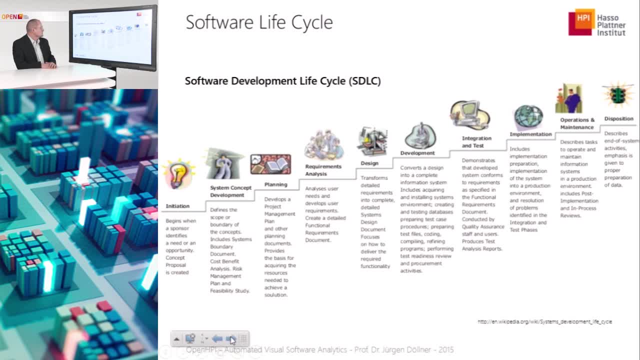 including its environment, creating and testing databases, preparing test cases, etc. Finally, integration and test when part of the system are already operational and we start to test it, to run the system Implementation phase, when things get done and ported to the real environment. 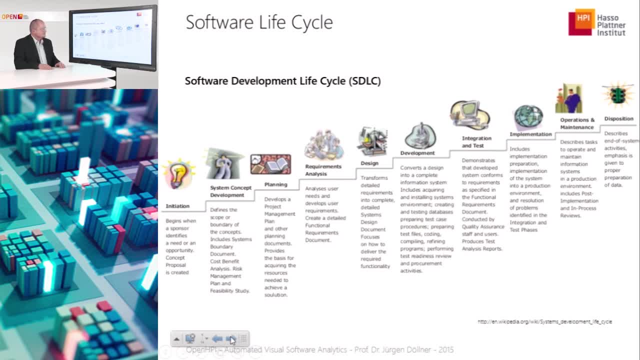 And operation and maintenance. It's in these large number of stages. It's the end, which describes tasks to operate and maintain information systems in a production environment, And finally, the disposition That's the end of a system when it gets retired. In this model, maintenance appears to be just one stage in the lifetime. 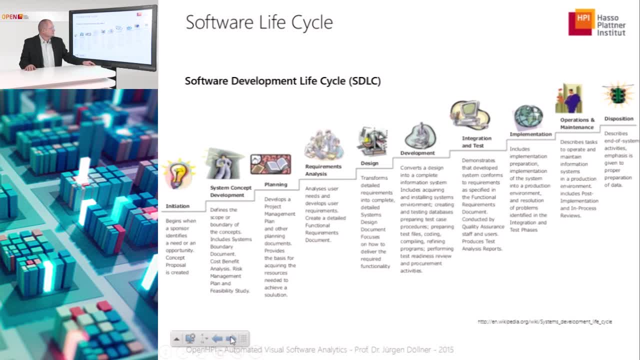 Reality is different. In reality, software maintenance, this part is a key part because it takes most likely many years, even decades. So while these are the stages, the stages done in the beginning of a system very intensively, somehow maintenance hides the fact that during maintenance, 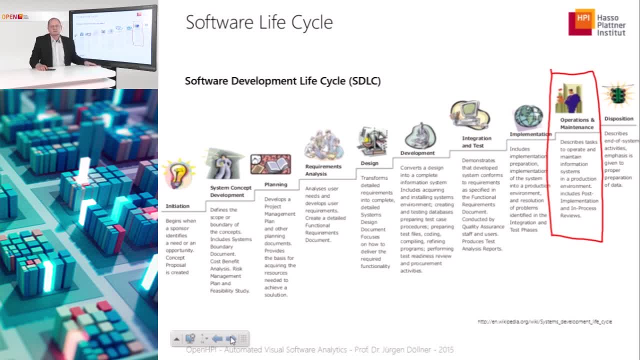 all these stages are repeated and repeated, Because maintenance means that the system evolves and evolution means that it's extended. So what we can see here in this model of the life cycle of a software system, that formally, operations and maintenance appear to be just one stage. 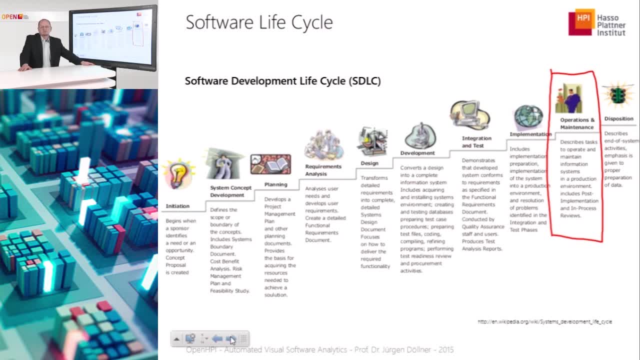 but practically, operations and maintenance represent key part, major part of the lifetime of a software system. So whenever we talk about methods, techniques, tools that improve software development, we should focus on the maintenance phase, because this is a major phase in the lifetime of a software system. 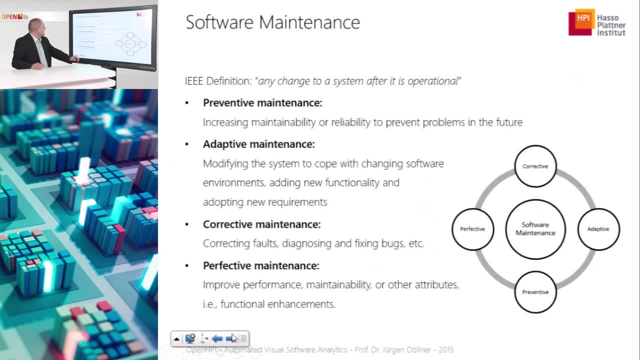 Let's go into details. What is maintenance? Maintenance is defined as the phase where you have any changes to a system after it became operational. Maintenance can be differentiated according to different goals, to different objectives that are behind maintenance activities. One key direction of maintenance is called preventive maintenance. 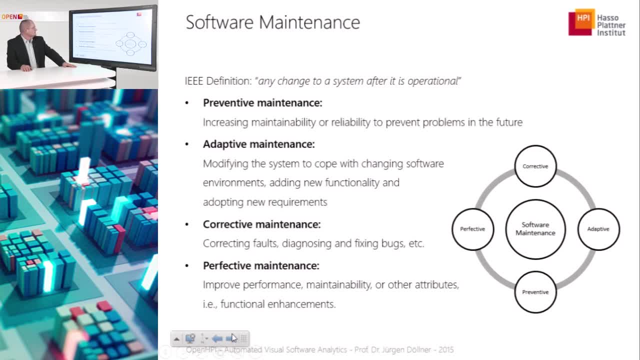 That means increasing the maintainability or reliability to prevent problems in the future, Maybe problems that did not already occur but say are likely to occur. So if we prevent problems in the future, if we, for example, increase software quality, then it's called preventive maintenance. 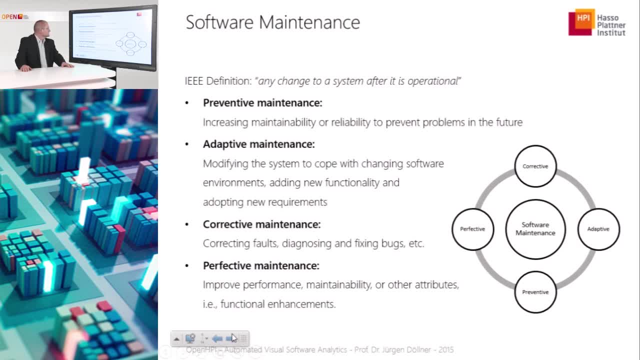 Another key dimension of maintenance is called adaptive maintenance. That means everything that is done to modify the system in order to cope with changing software environments, adding new functionality and adopting new requirements from the client or from customers. So adaptive maintenance is daily business in the evolution of complex software systems. 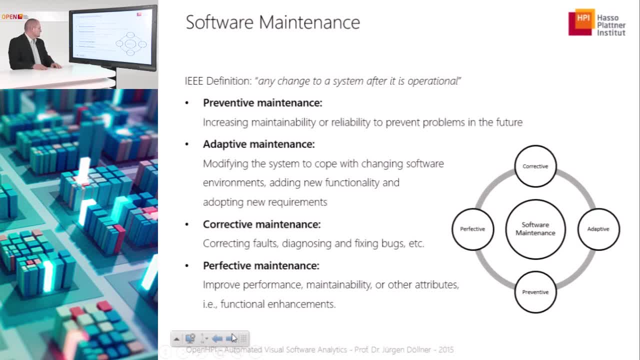 Corrective maintenance has a clear goal: It's about correcting faults, diagnosing and fixing bugs, etc. Whereas perfective maintenance aims at improving performance, maintainability or other attributes of software quality, including functional enhancements. Though what we see is that maintenance has different motivations. 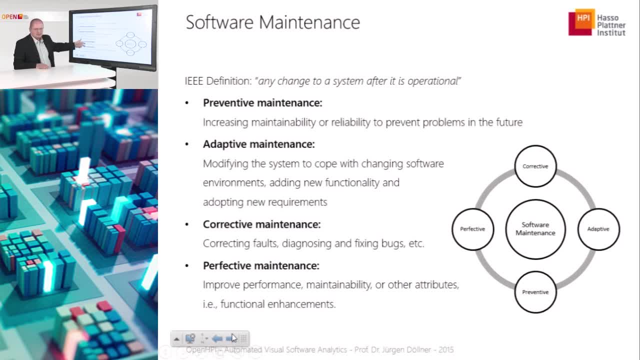 In reality, sometimes these motivations blend into each other. So you can never clearly differentiate between, for example, preventive and perfective maintenance, because sometimes, and in many real projects, these different aspects are merged and form a complex motivation to enhance a system. 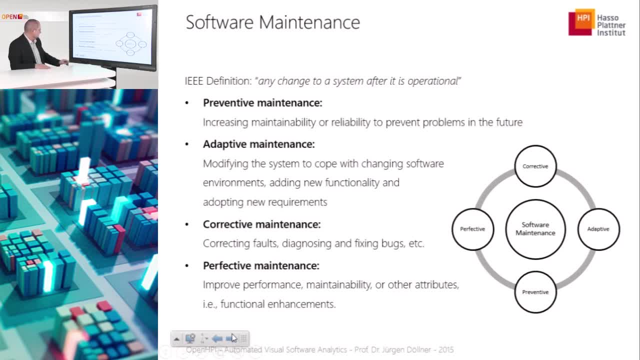 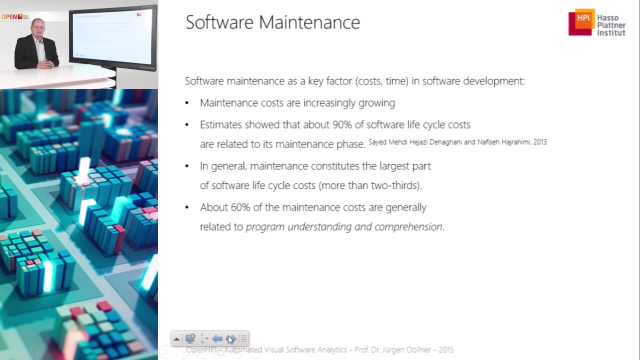 after it became operational. So that's software maintenance. And now the really interesting fact about software maintenance is that it's a key factor in terms of costs and time in software development. Maintenance costs are increasingly growing, especially if systems become aged, If we talk about legacy systems. 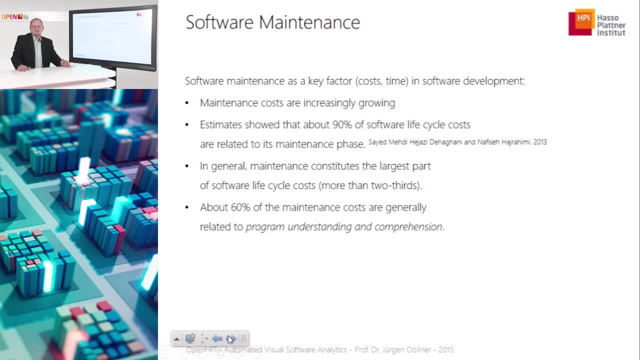 then the maintenance represents a major stage in the software lifetime. It's estimated that about 90% of software lifecycle costs are related to the maintenance phase. If we look at this fact, about 90% means that it differs according to the type of software system. 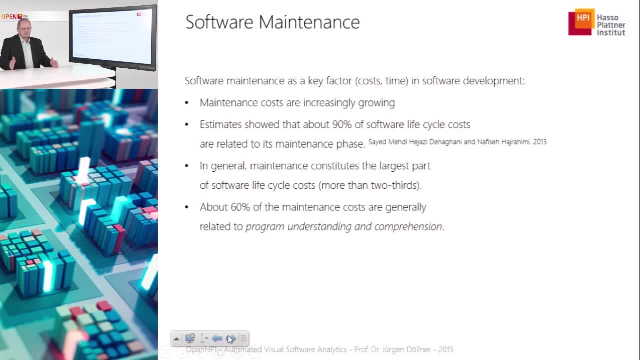 or the branch of the software system. it's the main, But more or less a major part of budget is spent for maintenance. But if we take this as a fact, then we can ask: well, do we have the right tools, techniques and methods? 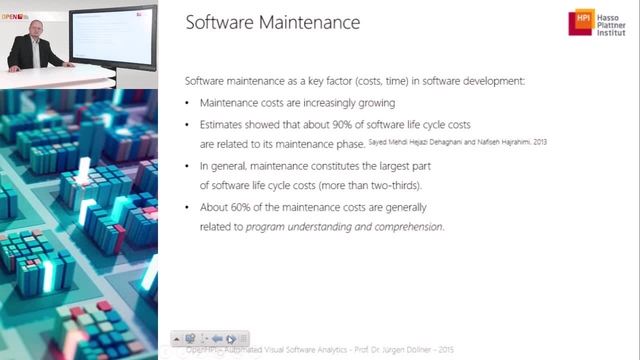 for software development if these tools, methods and techniques focus on the initial phase instead of the maintenance phase. What we will find out, and what we will explore in the other parts of this course, is that there is really a need for better tools and techniques and methods. 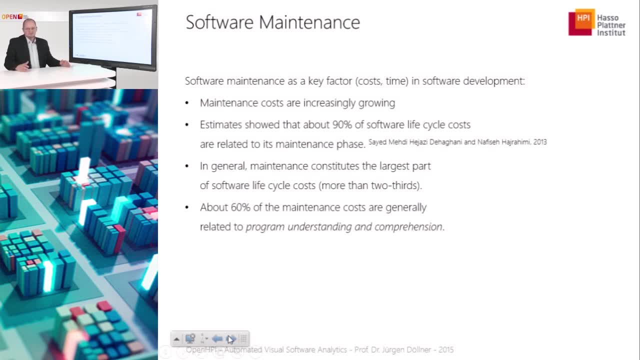 that handle and support the maintenance phase of software systems. This is maybe one of the key weaknesses of today's software engineering: that it's not really focused on the maintenance phase. However, if we look into the future, we can already foresee that maintenance. 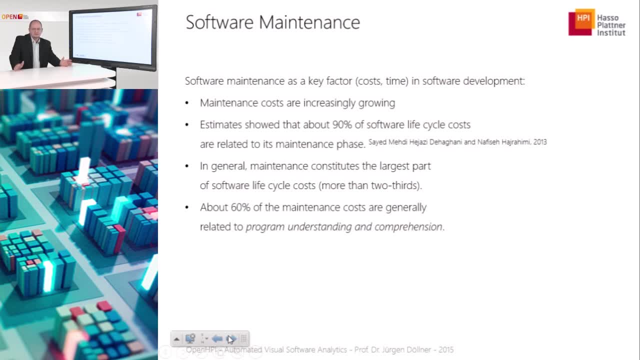 will become the central issue in software development. So in general, maintenance constitutes the largest part of software lifecycle costs- more than two-thirds- and about 60% of the maintenance costs are generally related to program understanding and comprehension. Program understanding and comprehension means. 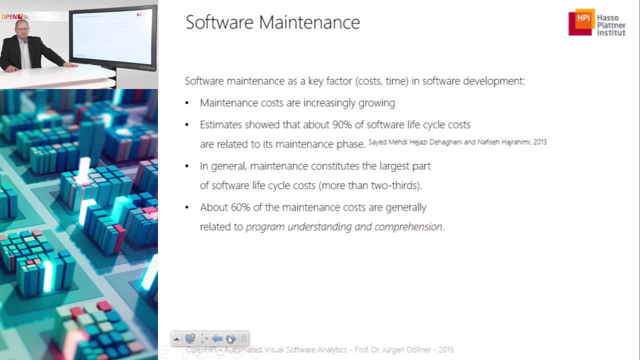 how can we get aware of a piece of the complex system? how can we enable developers to transform, to modify or to change that piece of the whole system? To do so, developers need to have information about this part they are dedicated to, And they have to understand and comprehend. 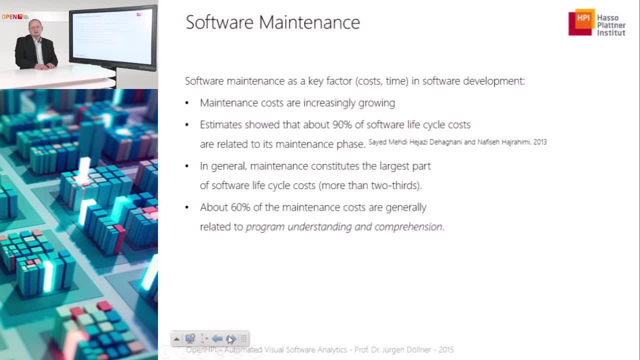 how it works. Think of having an old system and a new developer that starts to get involved. How can this developer become aware of the underlying models, dependencies, structures or behavior that is related to that piece he should, or she should, modify or transform? 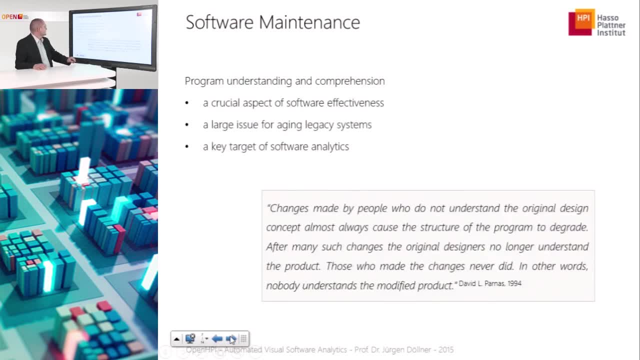 So program understanding and comprehension is a key issue. It's a crucial aspect of software effectiveness. So if we talk about how effective is our development process, program understanding and comprehension should be supported. It's a large issue for any aging legacy system. 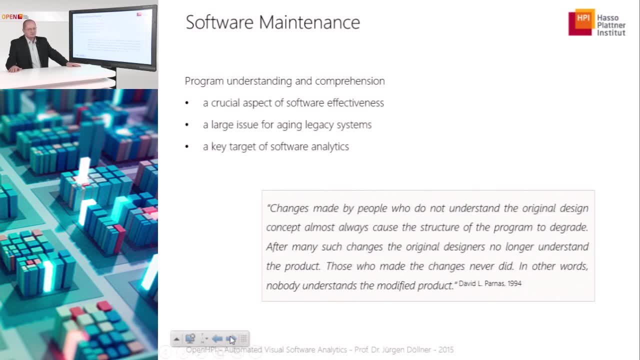 and of course, it's the key target of software analytics. The question for program understanding and comprehension has been investigated by a number of software engineer researchers in the past And, as David Parnas points out, change is made by people who do not understand. 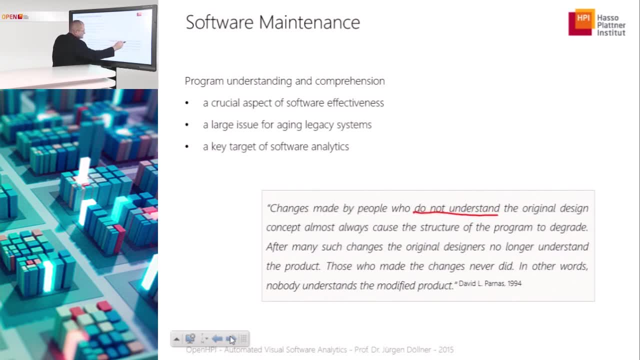 the original design, design and concept almost always cause the structure of the program to degrade. So if program comprehension and understanding does not take place, it is very likely that any changes and modifications done to the system will cause the software system to degrade After many such changes. 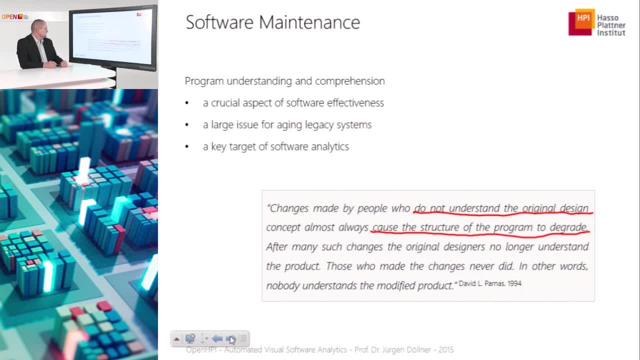 the original designers no longer understand the product. Maybe they are not anymore working for the company. Those who made the changes never did. In other words, nobody understands a modified product. So program understanding and comprehension represents a key issue for software maintenance. 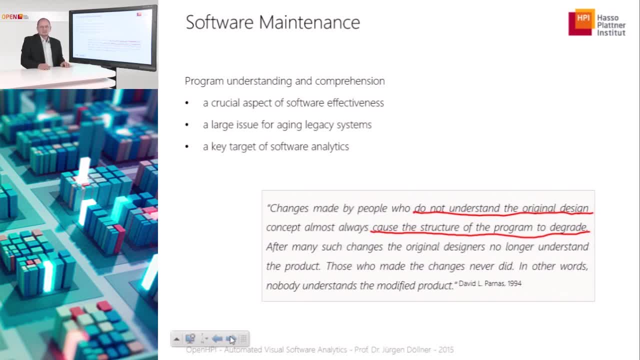 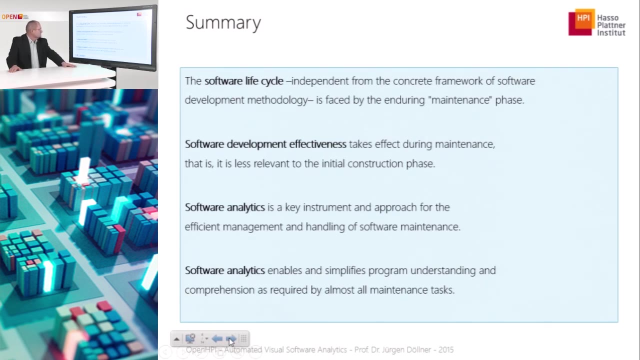 for effective software maintenance, and it's a key task to be supported by visual software analytics. Let's summarize the findings of this part. The software lifecycle is faced by the enduring, long-lasting maintenance phase And it does not depend from the concrete framework of software development methodology. 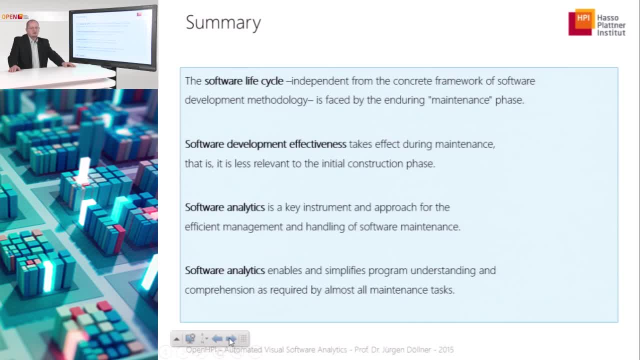 Whatever you use, you will have a long maintenance phase. if you develop, for example, a legacy system, or if you develop any complex software system, Software development effectiveness takes effect during maintenance, That is, it's less relevant to the initial construction stage. 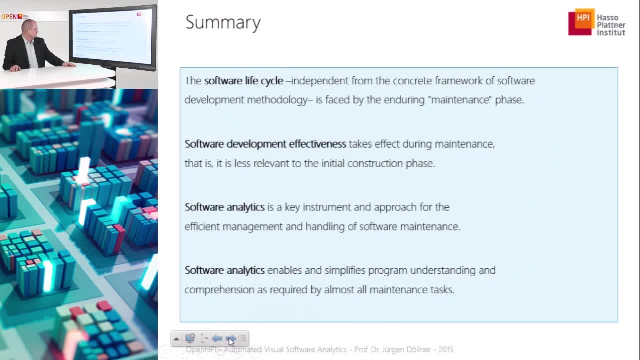 it's relevant to the maintenance phase. Software analytics is a key instrument and approach for the efficient management and handling of software maintenance. Of course it can be applied also to the initial phase, but its true value resides in the maintenance phase. Software analytics. 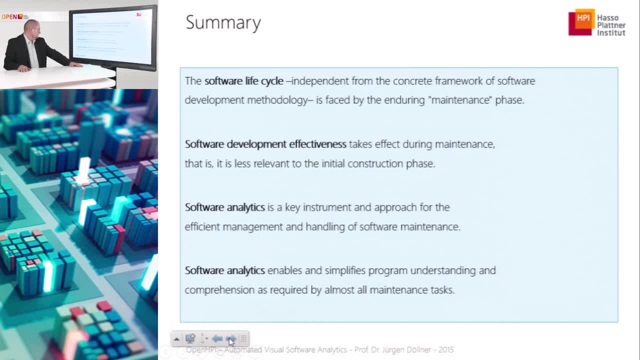 enables and simplifies program understanding and comprehension as required by almost all maintenance activities and tasks. So software analytics is a key instrument for all these issues we find during software maintenance, And software maintenance is in a sense, a reality of software development. Sometimes 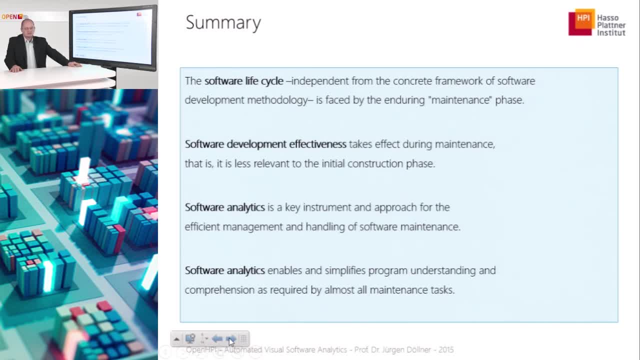 literature and science. it's not reflected too much and it's not seen like this. but if you look at the time spent in developments in industry, you find that software maintenance is a key issue there because it takes years. it takes decades. 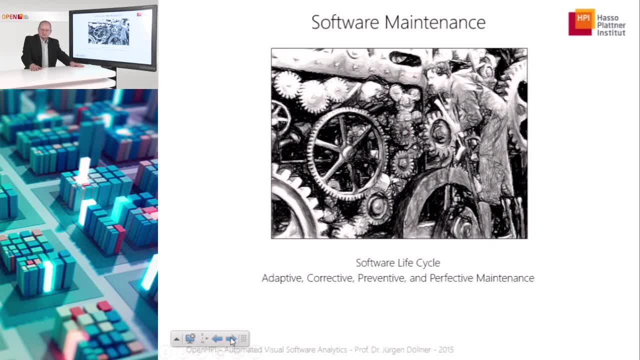 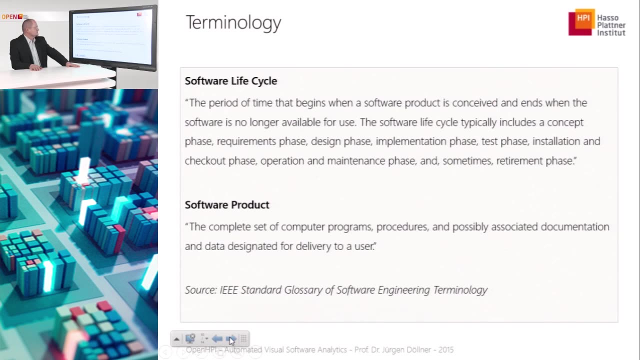 Let's summarize key terminology of software maintenance regarding the software lifecycle and adaptive, corrective, preventive and perfective maintenance. The software lifecycle is a period of time that begins when a software product is conceived and ends when the software is no longer available for use. 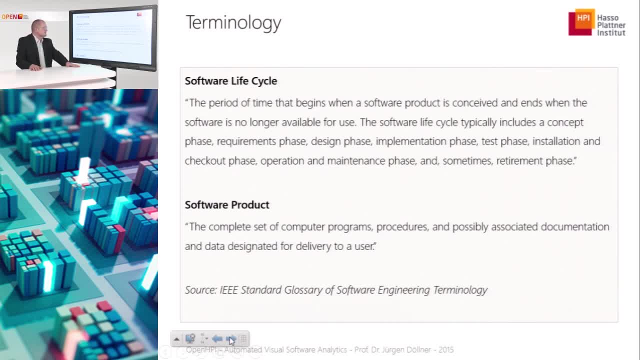 so-called retirement. The software lifecycle typically includes a concept phase, requirements phase, design phase, implementation phase, test phase, installation and check-out phase, operation and maintenance phase, and sometimes the retirement phase, According to the methodology, these stages that are described here. 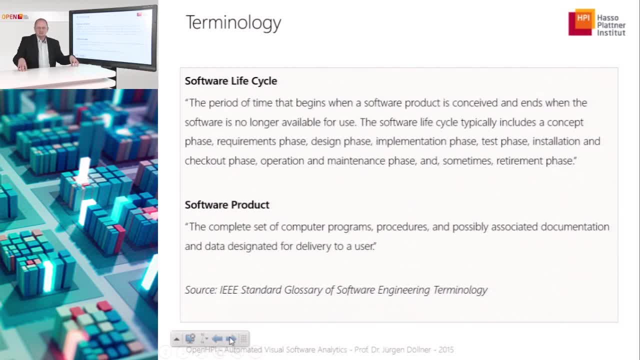 are arranged at a time where the software is in a state of access. If you, for example, use HR methods, then you have several iterations and these stages are repeatedly done. The software product represents a complete set of computer programs, procedures and possibly associated. 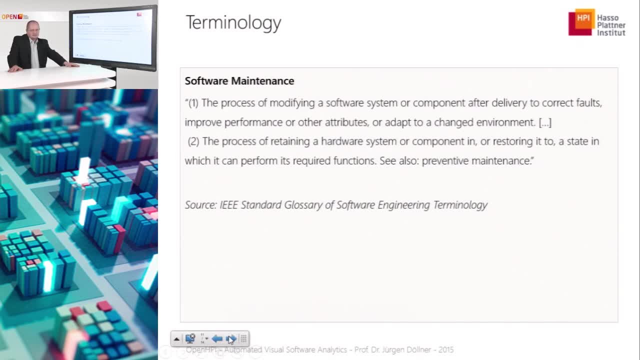 documentation and data design for delivery to a user. The software lifecycle is the process of modifying a software system or component after delivery to correct faults, improve performance or other attributes or adapt to a changed environment. The process of retaining a hardware system or component in. 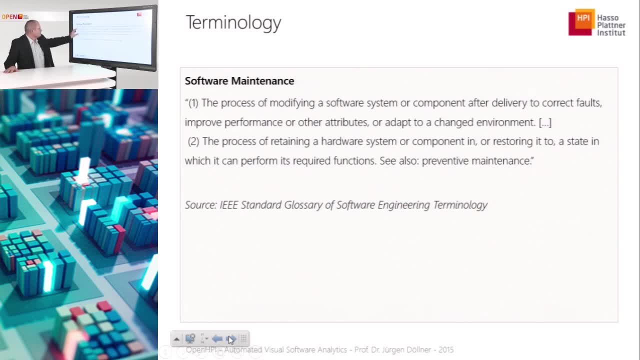 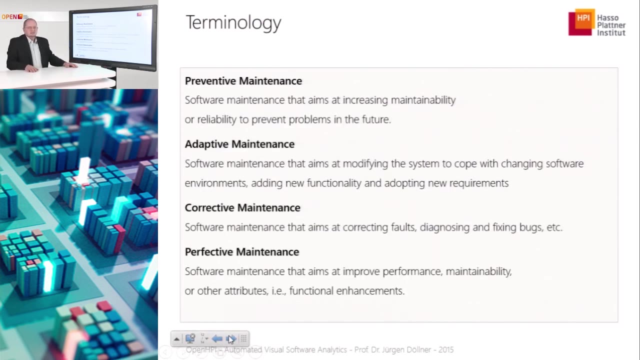 or restoring it to a state, is the first step in the development of a software system. Of course, we focus on the first definition because we talk about software systems, we talk about analytics for software systems. The second definition is to cope with changing software. 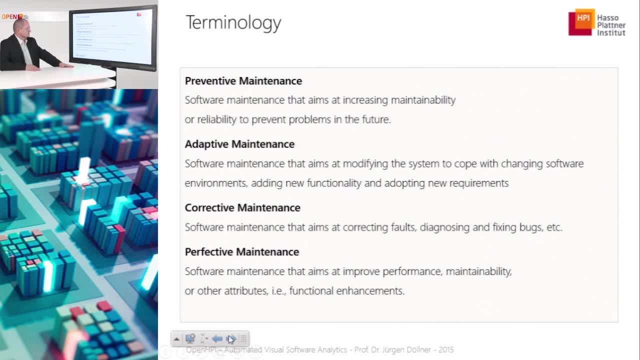 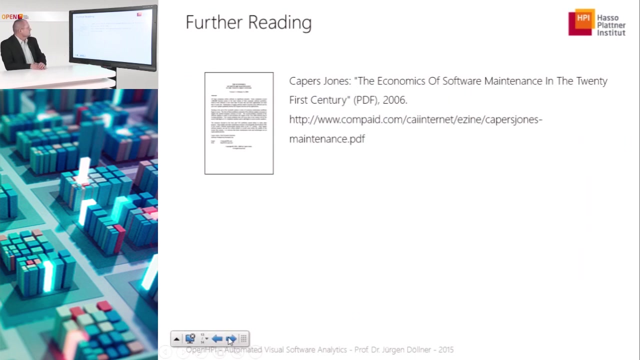 environments, adding new functionality or adopting new requirements. corrective maintenance that aims at correcting faults, diagnosing and fixing bugs. and, finally, perfective maintenance that aims to improve the performance of a software system. The third definition is to improve the performance of a software. 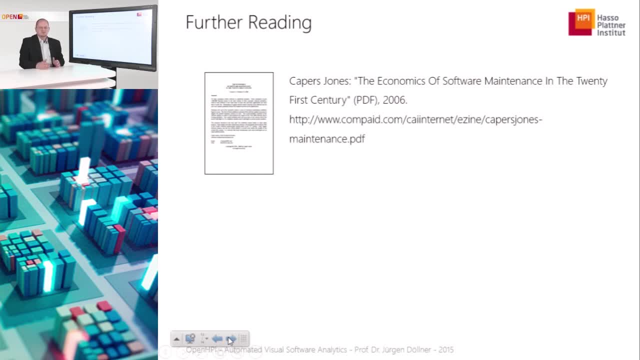 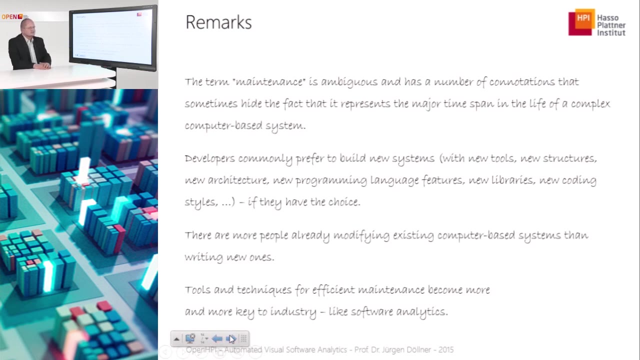 system. The third definition is to improve the performance of a software system. I also want to give you some remarks. The term maintenance is ambiguous and has a number of connotations. that sometimes hides the fact that it represents the major time spent in a software. 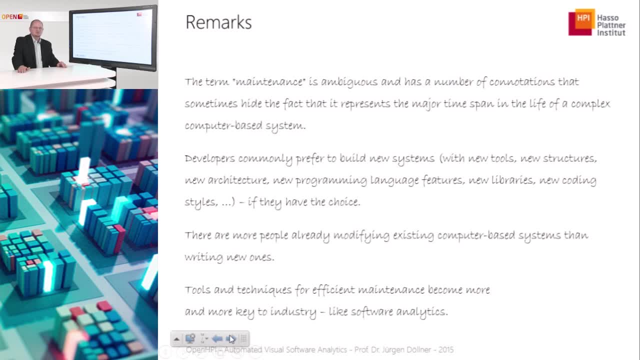 system. It is not considered to be a creative phase. Software engineering, however, software maintenance, is just the name for the long time after the initial construction of a software system. If developers would have the choice, if I would have the choice, I. 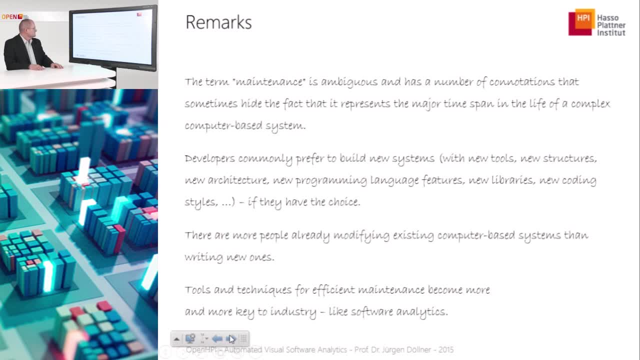 always would like to prefer to build a new system, selecting new tools, thinking about new systems, But that is sometimes a dream, because if we start working in a big company, most likely we will not have the chance to create a new system from.